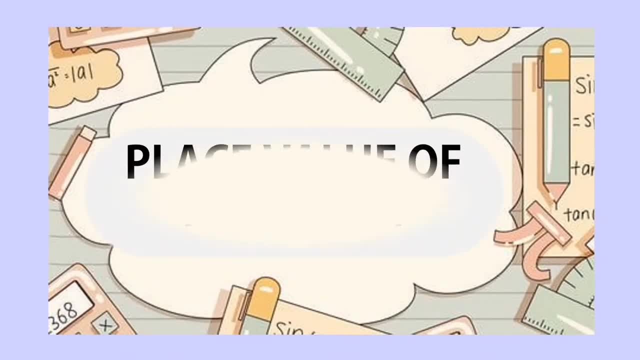 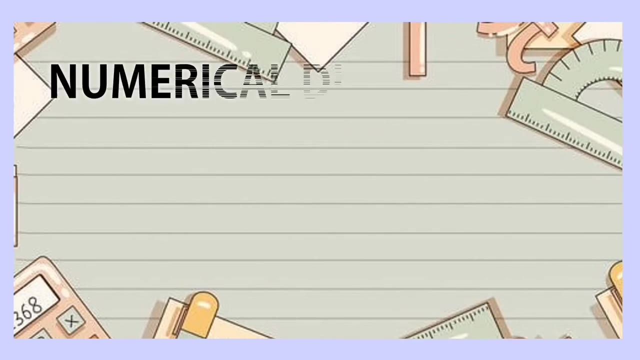 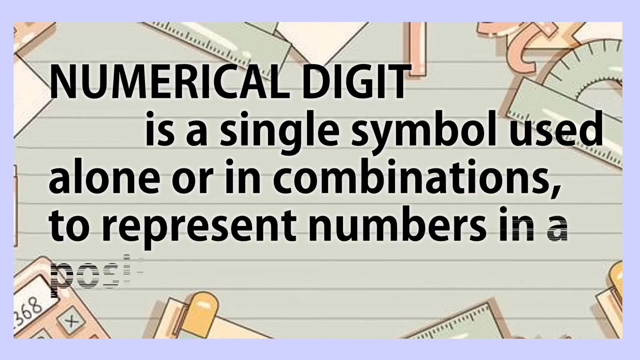 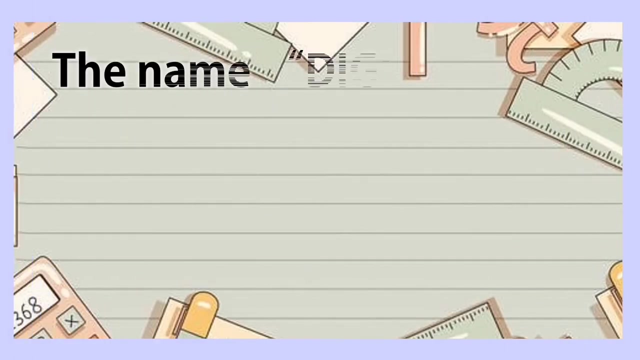 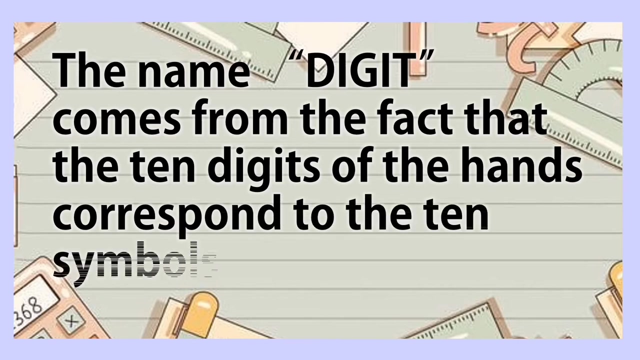 Place value of a number. Before we go to the main topic, which is place value, let us first define the following terms. Numerical digit: It is a single symbol used alone or in combinations to represent numbers in a positional numeral system. The name digit comes from the fact that the 10 digits of the hands correspond to the 10 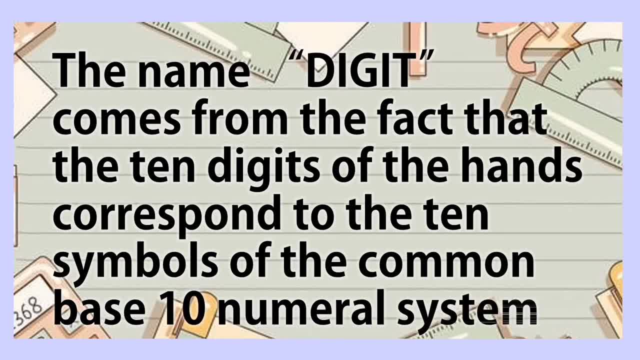 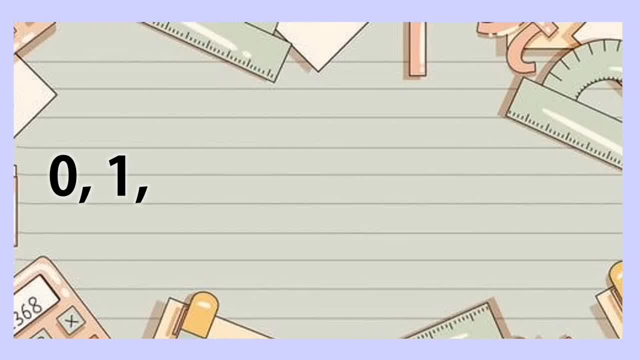 symbols of the common base 10 numeral system. These are 0,, 1,, 2,, 3,, 4,, 5,, 6,, 7,, 8,, 9,, 10,, 11,, 12,, 13,, 14,, 15,, 16,, 17,, 18,, 19,, 20,, 21,, 22,, 23,, 24,, 25,, 26,, 27,, 28,, 29,, 30,. 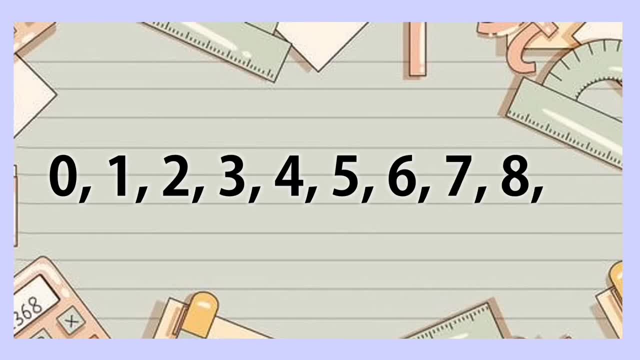 30,, 31,, 32,, 34,, 35,, 36,, 37,, 38,, 39,, 40.. So these are the 10 digits composing the base 10 numeral system. Now let's take a look with these digits. 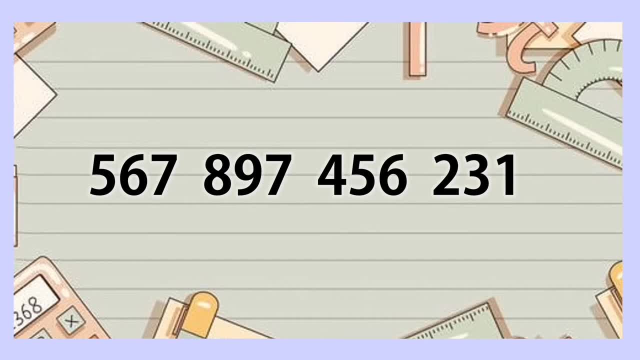 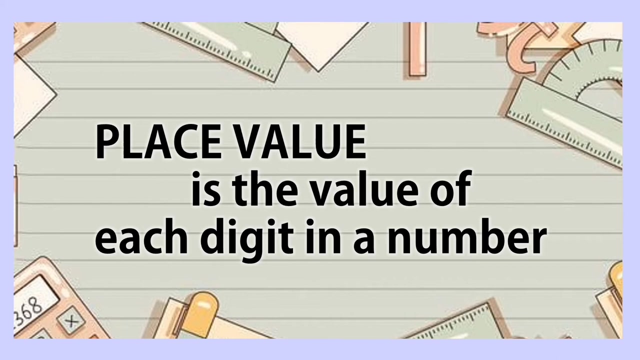 Digits are divided into periods and normal periods. Normally, each period contains maximum of three-digit numbers. Every period is separated by a comma or a space, So now we can read it as 567,897,456,231.. Now let's proceed to place value. Place value is the value of each digit in a number. 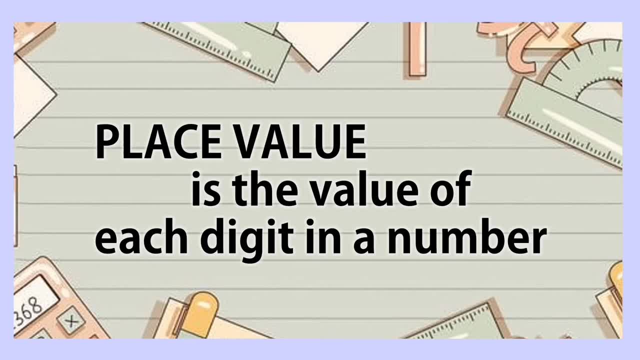 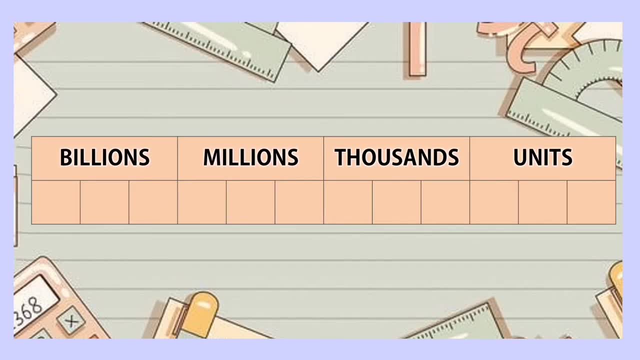 Each digit in a number has its own value depending upon its position in the place value chart. So this is a place value chart. Here we have four periods, which are units, thousands, millions and billions. Now let us determine the value of each digit in this numeral. 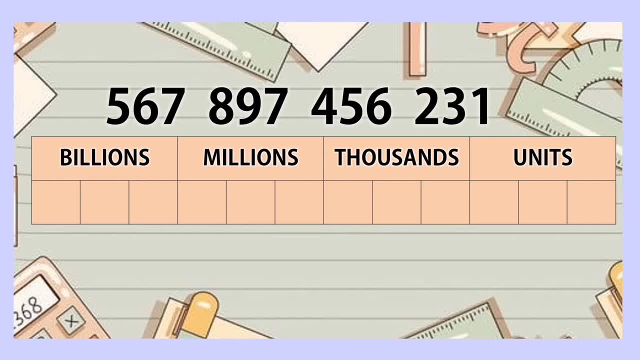 So let us place this in the place value chart. Let us start from the left. So we have 1,, 3,, 2 in units period, 6, 5, and 4 in thousands, 7, 9,, 8 in millions and 7, 6, 5 in billions. 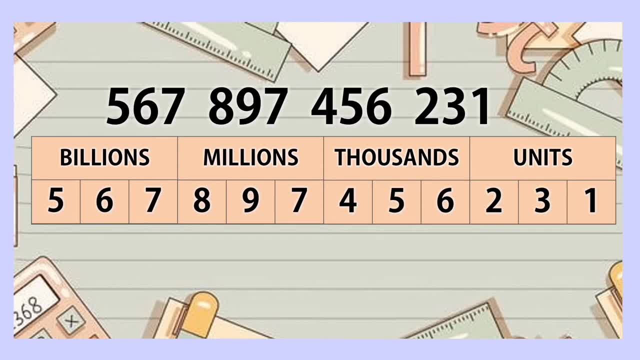 Now that we have already placed the digits inside their corresponding boxes, let us now identify the place value of each digit Again. let's start from the left. So in units there are ones, tens and hundreds place value. So the place value of one is ones, three is tens and two is hundreds. 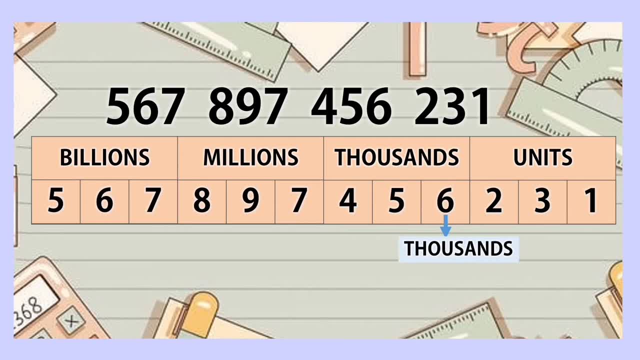 In thousands we have thousands, Millions, ten thousands and hundred thousands, So the place value of six is thousands. five is ten thousands, four is hundred thousands. In millions we have millions, ten millions and hundred millions, So the place value of seven is millions, nine is ten millions and eight is hundred millions. 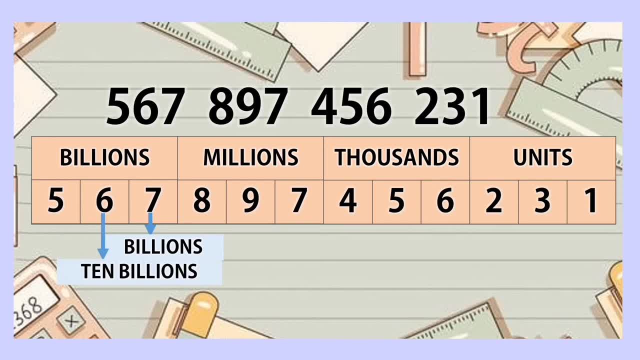 In billions. we have billions, Billions, ten billions and hundred billions. So the place value of seven is billions, six is ten billions and five is hundred billions. Again, digits are divided into periods. These periods are units, thousands, millions and billions. 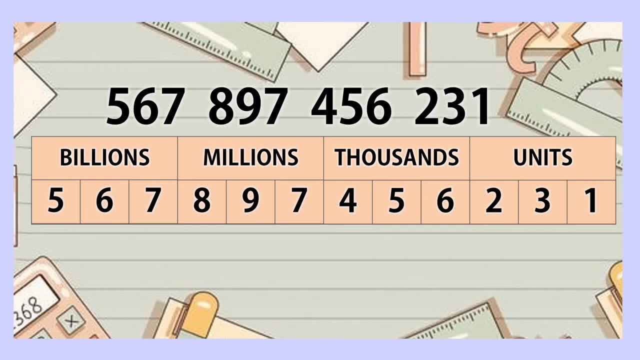 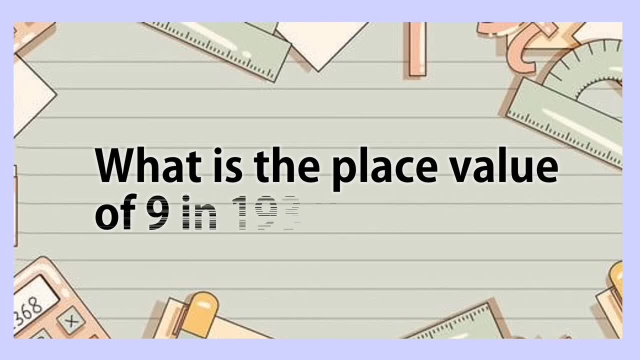 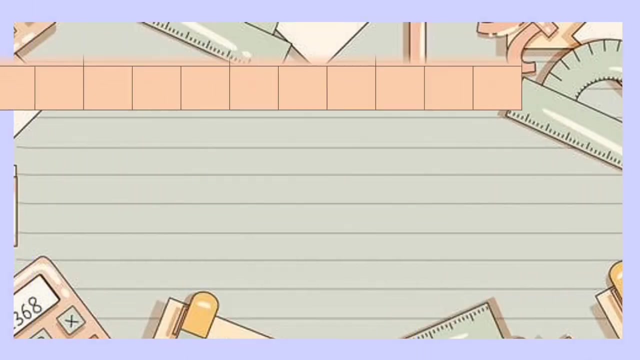 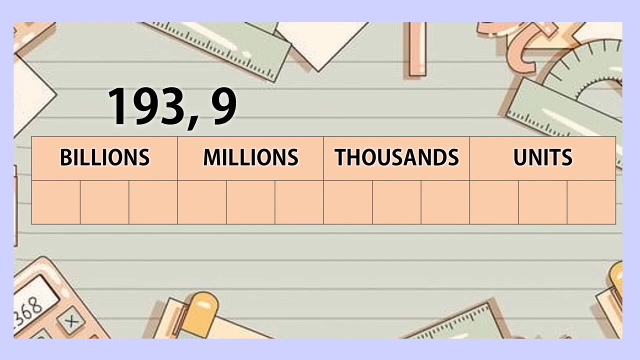 To deeply understand this lesson, let us solve few examples. What is the place value of each nine in the number shown? So here we have three nines. To determine the answer, let's place this number inside the place value chart. Let's start on the decimal.